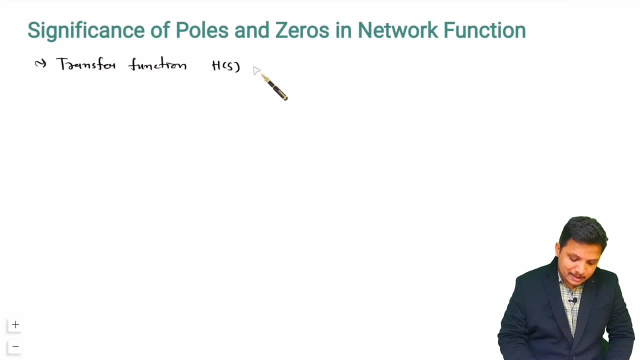 transfer function is H of S, that is output C of S divided by input R of S. Now I'm just assuming one transfer function with polynomial. So in numerator if I say I'm having A N S to the power n plus a n minus 1 s to the power n minus 1, plus up to a 1 s to the power 1 minus 1, 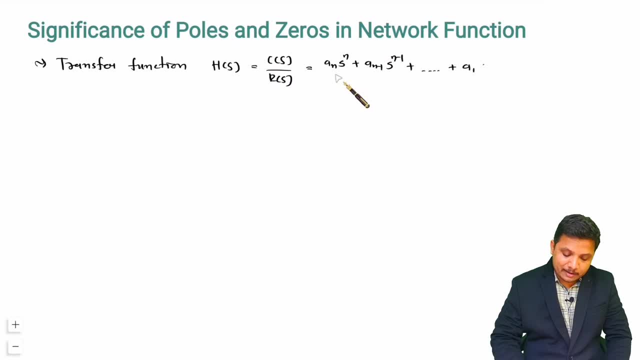 means s to the power, 0 means a 1, right. Similarly, with denominator. let us say we are having b m- s to the power m plus b m minus 1, s to the power m minus 1 plus up to b 1.. See, this is how. let us say we have two polynomial: One is numerator polynomial and 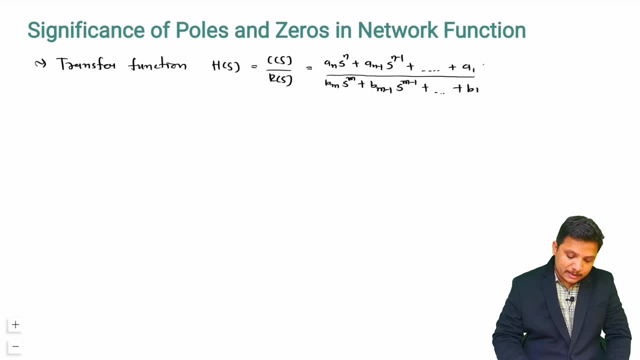 second is denominator polynomial. So, my dear students, if you observe numerator polynomial, which is having power n right, And if you observe denominator polynomial, that is having power n right, So you can see that we are having b m s to the power m plus, b m minus. 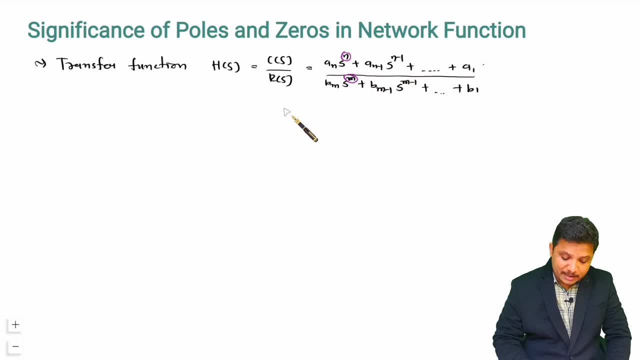 m. So what it means? It means that for numerator, polynomial power n is there, which means there are n number of zeros in this transfer function. So power n in numerator explains there are n number of zeros and if you observe denominator, that is having power m. So what it explains. 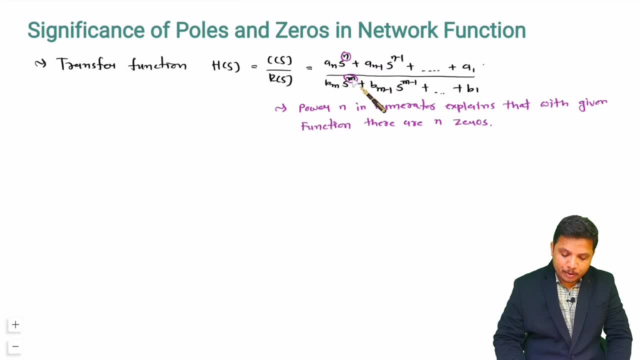 It explains that there are m number of poles. So see: numerator polynomial's power explains number of zeros and denominator polynomial's power. that explains number of poles. right Now, my dear students, what I will do is I will explain you. transfer function by location of. 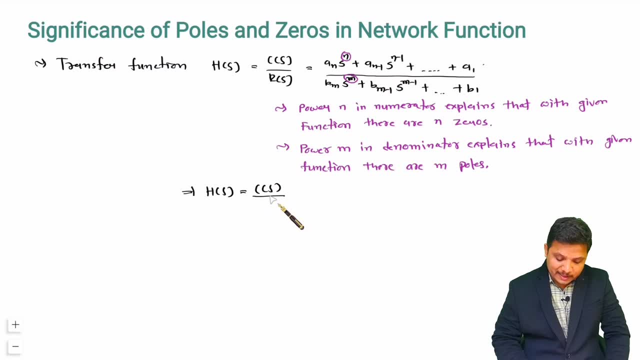 poles and zeros. So, as I have told you, transfer function is a function of the number of zeros. So a function is what Output divide by input, right? So if transfer function that is given in terms of roots, right, Like you see here, numerator polynomial is having s to the power. 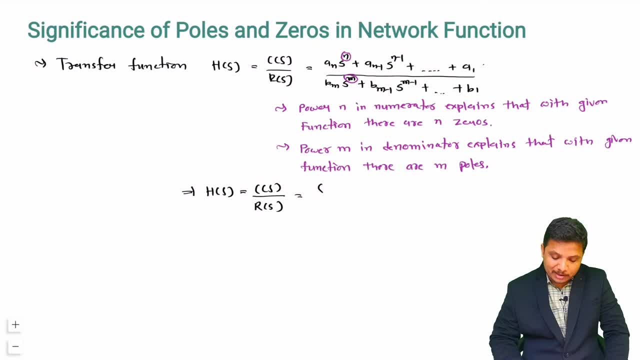 n power. So how many roots will be there? with numerator polynomial, There will be n roots. So let us say s minus z 1, s minus z 2, up to s minus z n number of roots are there with numerator polynomial and with denominator polynomial, it defines poles right and here. 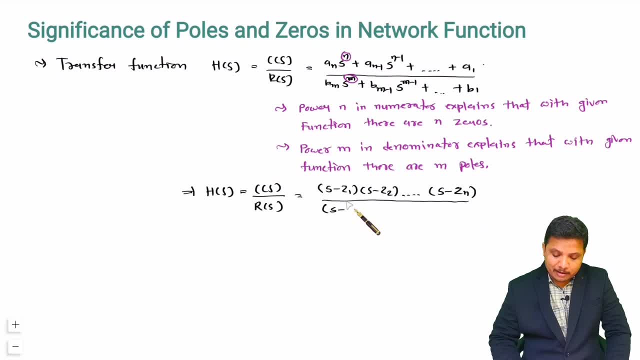 power is m. so let us say there are m number of roots. those are like s minus p1, s minus p2, up to s minus pm. then you see these roots. that explains location of zeros and poles, right? so see these zeros and poles, locations that we can identify by having roots of polynomial. 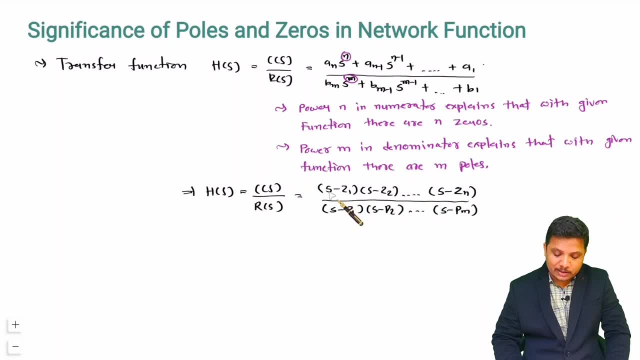 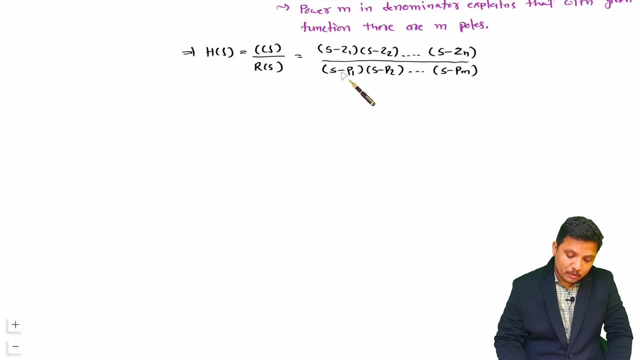 numerator polynomials roots will identify location of zeros, and denominator polynomials roots. that will identify locations of poles. right now, my dear students, i'll explain you how to identify stability. so for stability, identification, location of poles are very essential. now to explain you stability, you see, this is imaginary axis. 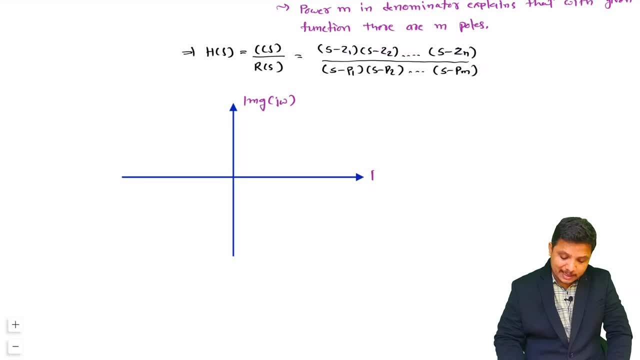 which is j, omega, and this is real axis, which is sigma. now, how to identify stability? so here you just observe, this is left half plane and this is right half plane and this is imaginary axis, right delle right. in that case we can say: system is system is marginally stable, and see at origin. here we have center at origin, if we have one. 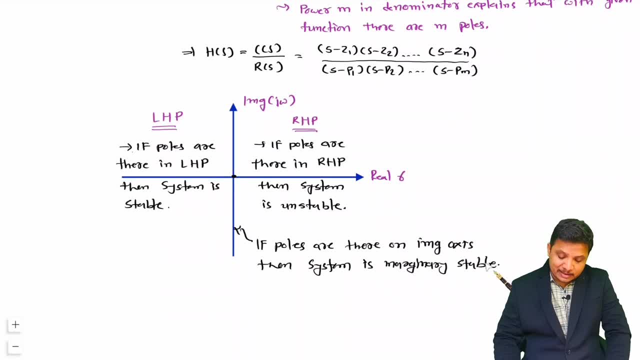 pole, then you can say system is marginally stable. but if you have more than one pole at origin, then system will be unstable. so locations of poles and zeros, that plays essential role to understand whether given system is stable or not. right? so, my dear students, first of all you will have to identify location by identifying roots. numerator roots are: 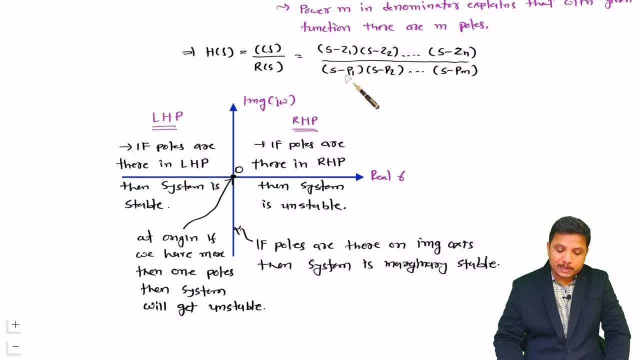 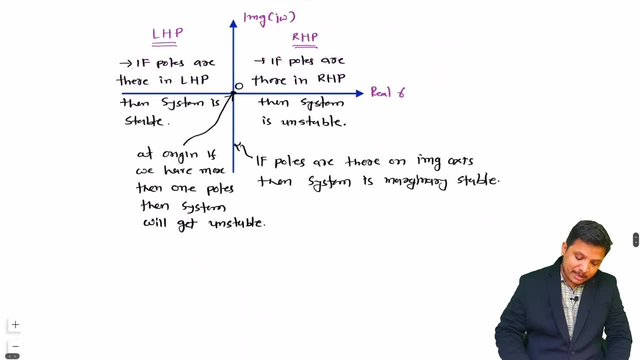 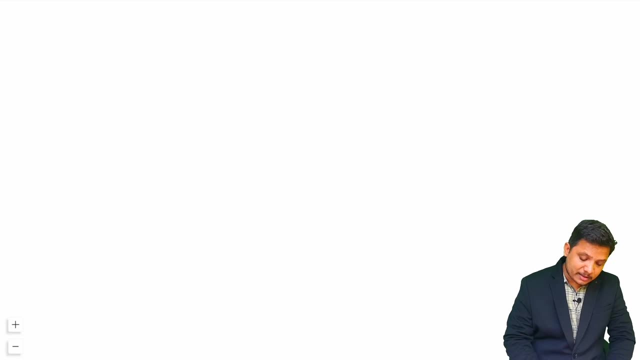 giving you location of zeros and denominator roots are giving you locations of poles. right now i will give you some examples so that will be giving you clear idea about how to identify stability for system. so let me write one question here first. now here we are given with function f of t, that is, e to the power minus t right, and question is to identify: 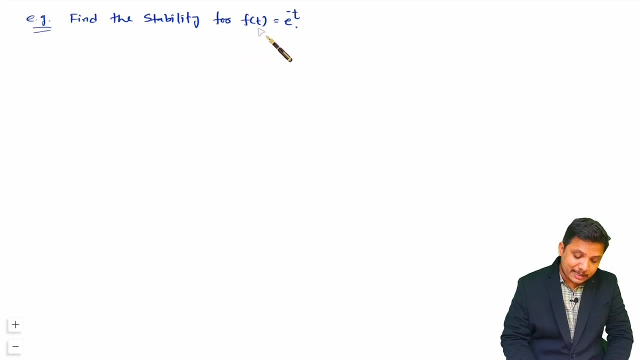 stability. so i will explain you stability calculation in terms of time domain as well as in terms of laplace domain. so what is happening in bounded region? right, so we can say system is stable. but it is very easy to identify that in terms of frequency domain. you see this f of t, that is, e to the 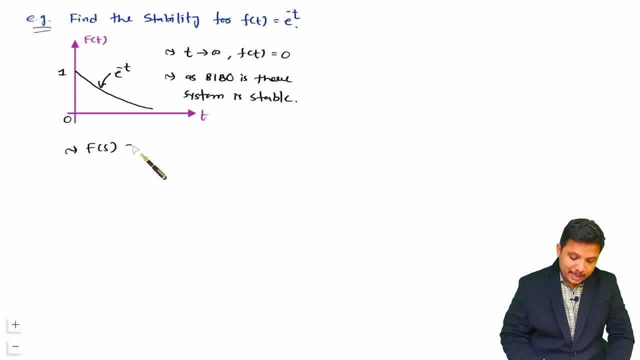 power minus t. so in laplace domain e to the power minus t will be one divided by s plus one right. so you see what you can say: is here denominator is having one root? and then you will say: is here denominator that is edgeÚ is going to be point one've got. 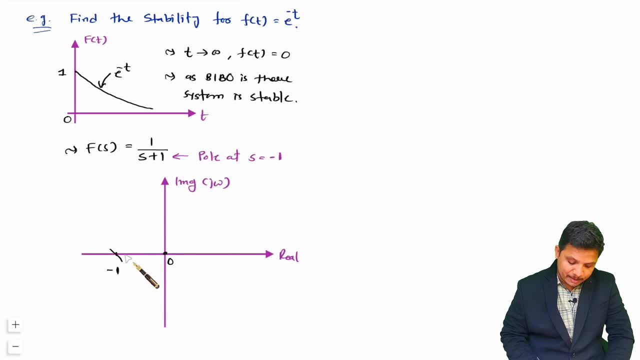 control and control f in particular, as James prônani said, respects decentralization. so that is changing other terms, right so? and if you observe that, well, right, we know, that is identifying pole. right so, pole is there at s, equal to minus one, right so if you observe that in this plane, then you'll see this is origin and s is equal to minus. one is having pole, so you should represent pole at s equal to minus one, and pole is represented by cross symbol. right now, you see one pole that is there on s plane, so here we can. now you see one pole that is there on s plane, so right. energy Marriage smooth Code. right now you see one pole that is thereедjae 20 têm, where geaje is thereappearance and activity. the important factor value is to be that our solar elements will happen. we can now assign to the influence- ничего aconteceu- with the time we want. 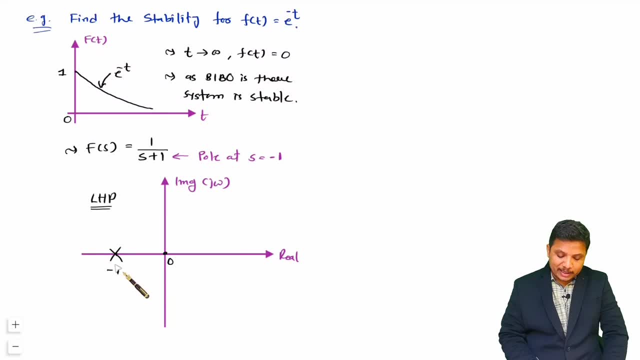 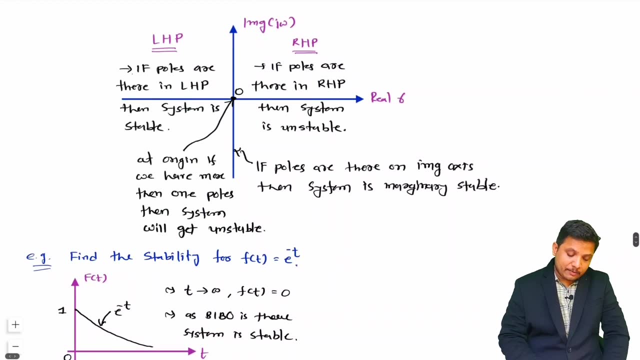 LHP right, left half plane. so what it indicates: this system is stable, right? I have already explained. you see, if poles are there on left half plane, then system is stable. if it is there on right half plane, then system is unstable. on axis it is marginally stable and at origin, if more than 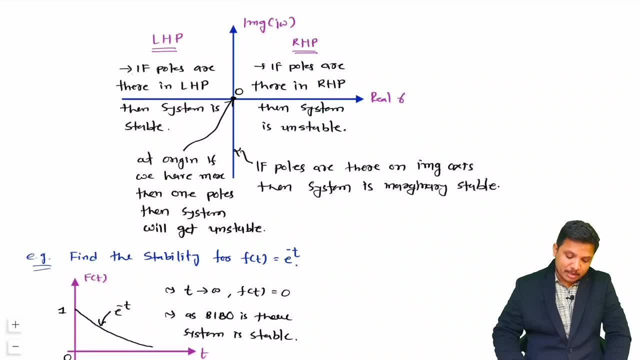 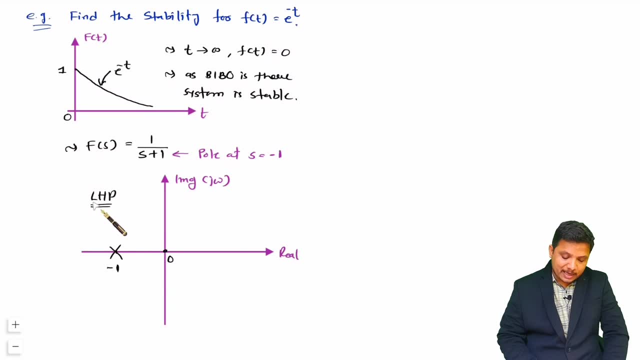 one pole is there, then system is unstable. so based on this you can say: system is stable as per pole is there. on LHP, let me give you one more problem. so this will gives you more resolution. now I am taking simple problem to explain you the concept. right? so here f of t, that is e to 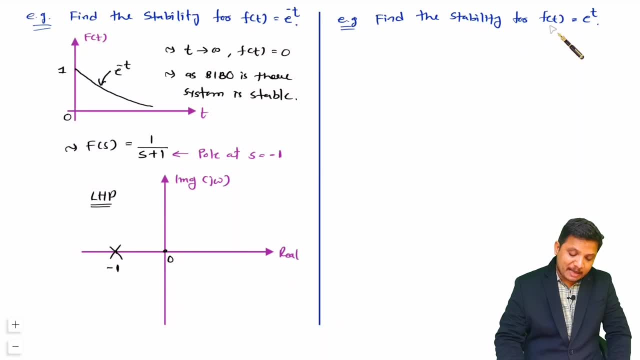 the power t that is given. so let us plot that in time axis first. so you see, f of t is e to the power t. so at 0 it will be 1. at time T is equals to 0, it will be 1. and you see, as time increases, it will increase exponentially. right, it will increase exponentially. 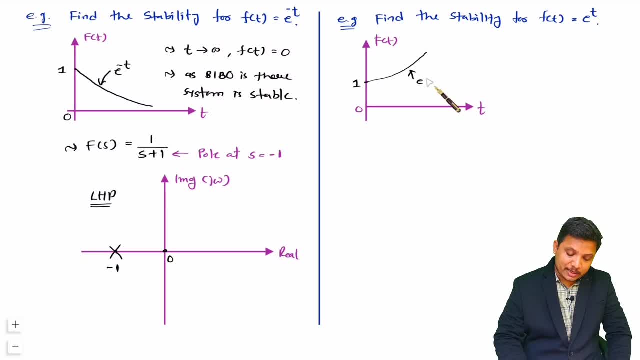 like this. so this is exponential function e to the power t. now you see what will happen, as if time T is going towards infinity. what will happen? this function f of T that will go to its two vertices and vice versa. right, or you can see, if f implementation. let me show you how to. 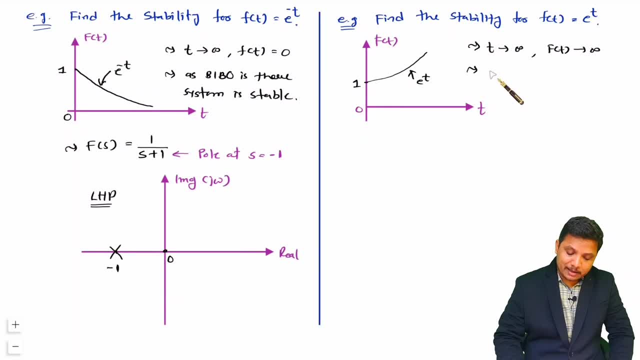 add two vertices together. so if f is equal to x, someone will start to propagate this function. then infinity right. so you can say: it does not give you bounded input, bounded output. why the reason is: output is going towards infinity. so you can say: we don't have bounded input, bounded output. so system is unstable. now, my dear students, 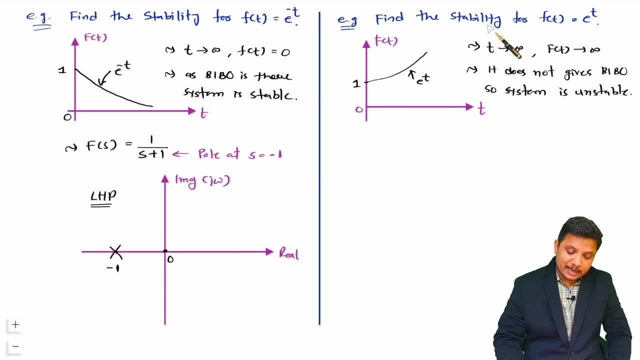 if you want to identify stability in terms of Laplace domain, then you see, it is quite easy. Laplace domain of e to the power T, that is 1 divided by s minus 1 right. so based on denominator we can identify location of pole, and pole is: 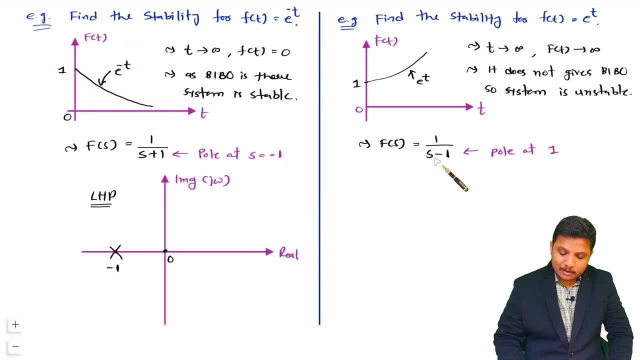 there at 1. right root is there at s is equals to 1. so I can say pole is there at 1. so if you plot that on s plane then you can see that it is quite easy. Laplace domain of e to the power T, that is 1. 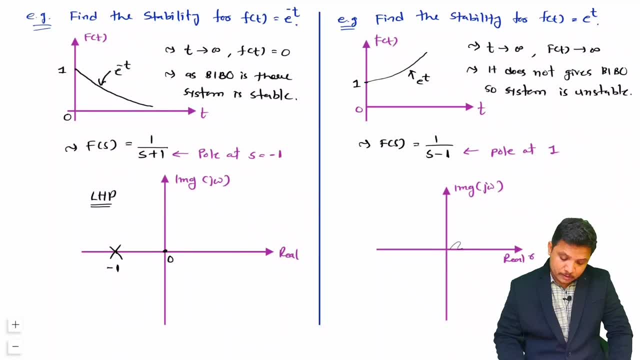 you can identify stability. so you see, this is origin, this is real axis. here we are having 1 and pole is there at 1, so here pole is there. so by cross symbol I should represent pole and you see this pole that is there on our HP right half. 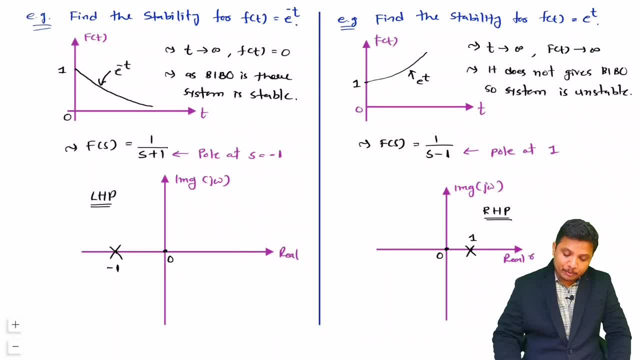 plane. so for right half plane, if any pole is there, you can say system is unstable, right. so see, in time domain we need to find functions range, but in Laplace domain, by just identifying location of poles, we can identify stability of the system. so, my dear students, it is very easy to analyze. 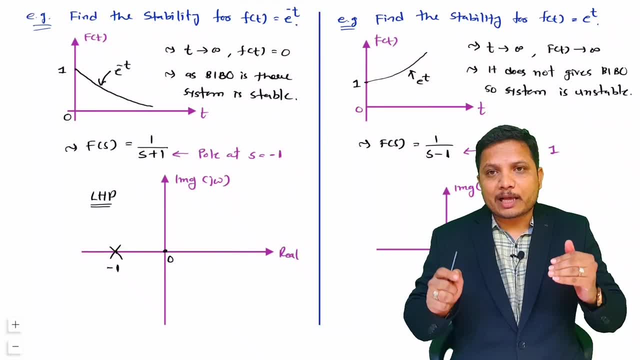 systems response. by using Laplacian function and by observing location of poles and zeros, we can understand stability of the system. so that is what the main significance which is there with poles and zeros in functional stability. I hope you have understood this. Thank you so much for watching this video.